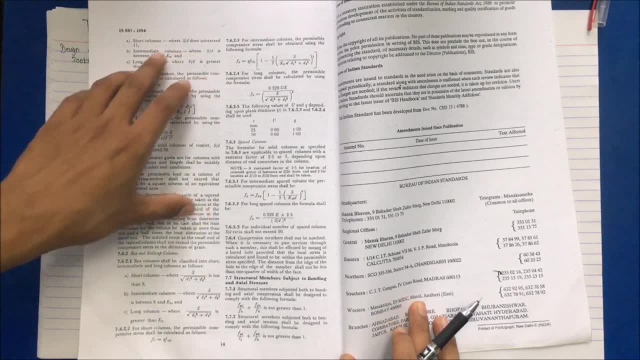 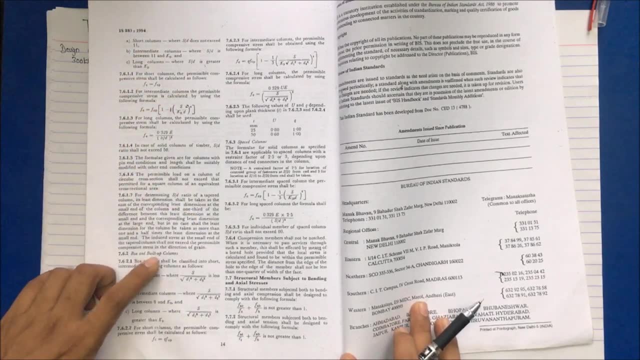 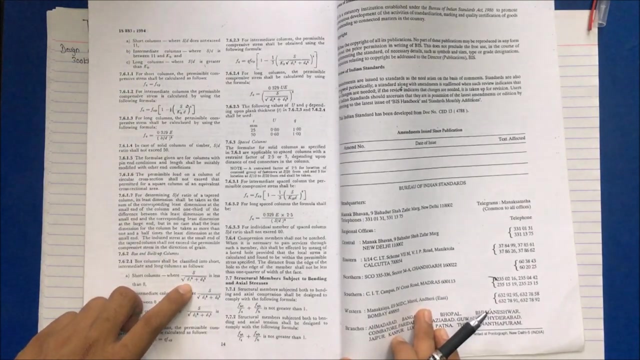 span of the column, and D is the depth, and this value is determining whether the column is short, intermediate or long. in case of box or built-up column, you will see a new term introduced here: D 1 and D 2. these are the values, or these are D 1 and D 2? okay, you can find it. what? 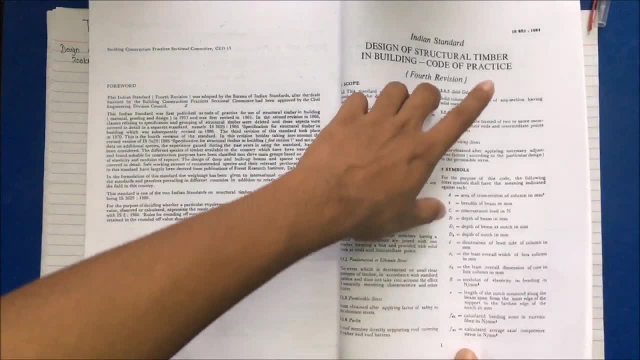 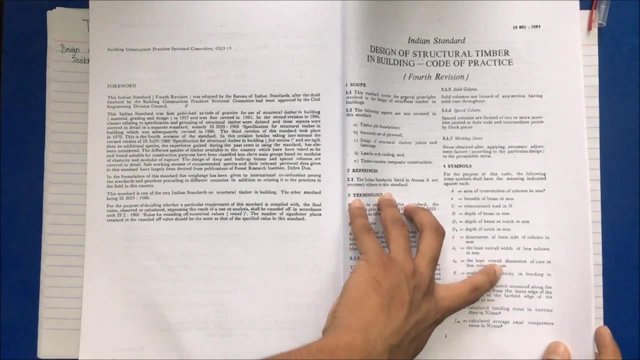 does it mean at page number 1 of is 883, so small D 1 and D 2. D 1 is the least overall width of the box in mm and the least overall dimension of core in box in mm. so these are the two dimensions of the box in mm. so these are the. 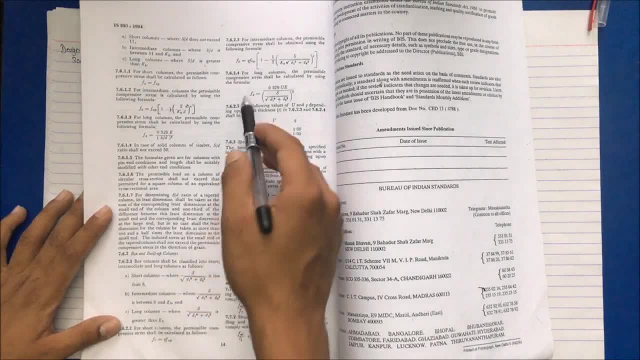 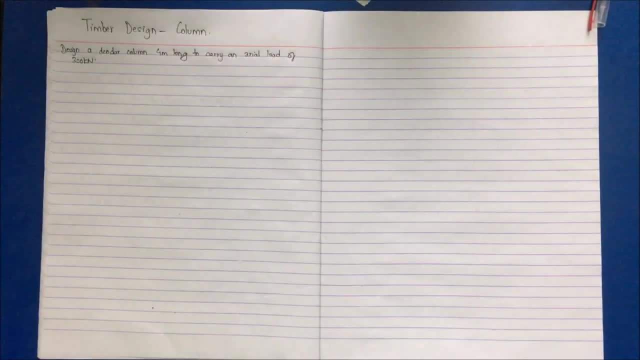 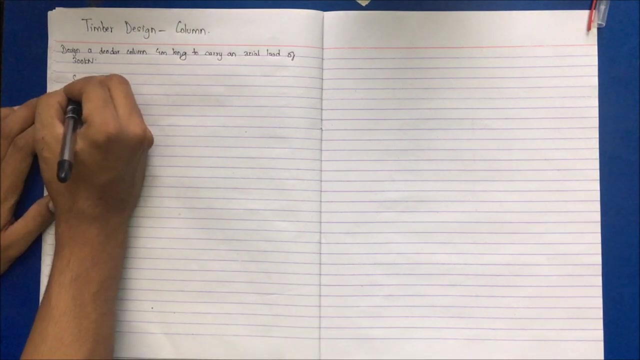 terms you have to understand. so these are the condition to satisfy whether the beam is short, intermediate or long column. now I have a question here. design a deodorant column 4 meter long to carry an axial load of 300 kilo Newton. so the design procedure you will be same for various. 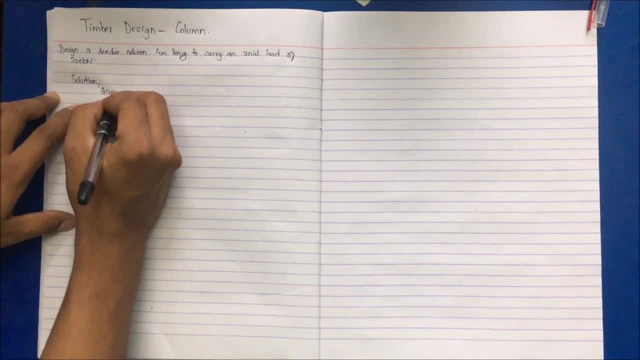 types of question. given area has to be calculated first. okay for this. I will be using the same procedure for the other two types of question. given area has to be calculated first. okay for this area has to be calculated first. okay for this area has to be calculated first. okay for this. 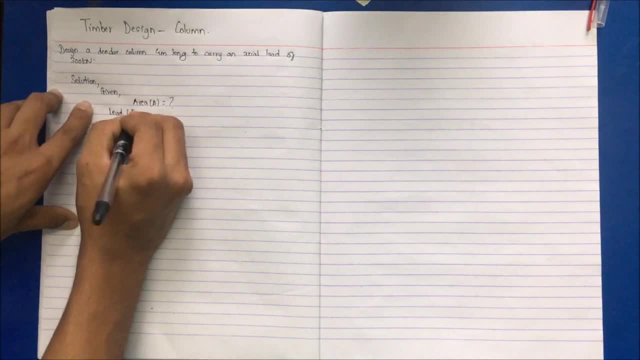 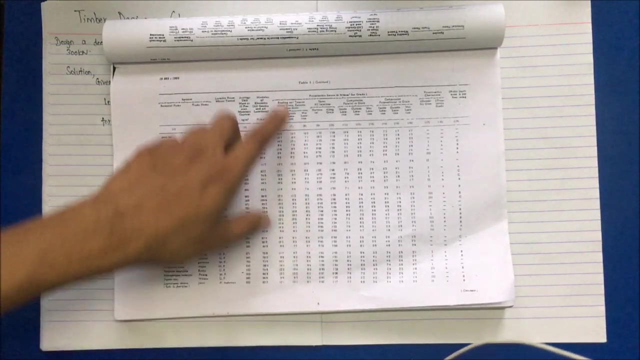 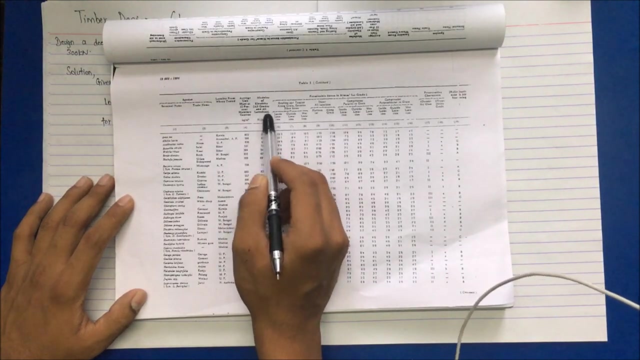 I have been given the load, 300 kilo Newton, and for deodorant column. so for deodorant, okay, we have at page number 9 of table 1 I find the values for average unit mass modulus of elasticity. okay, so deodorant of himachal pradesh row will be. 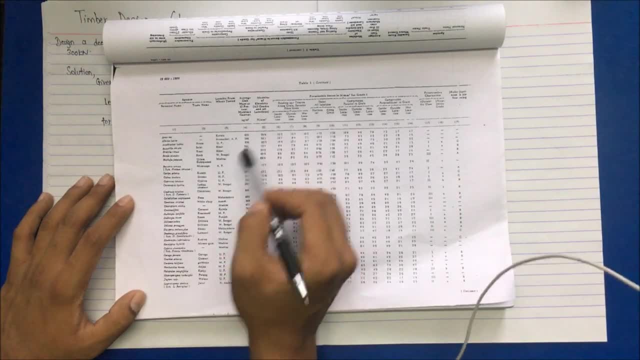 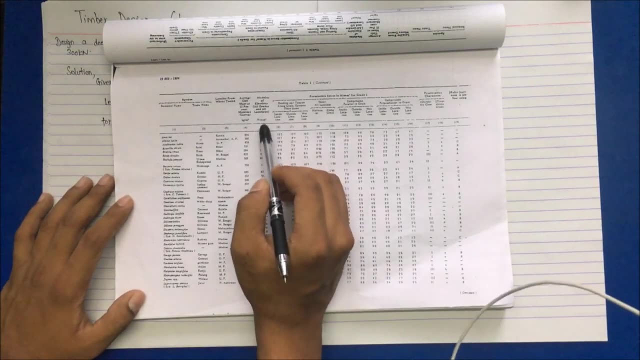 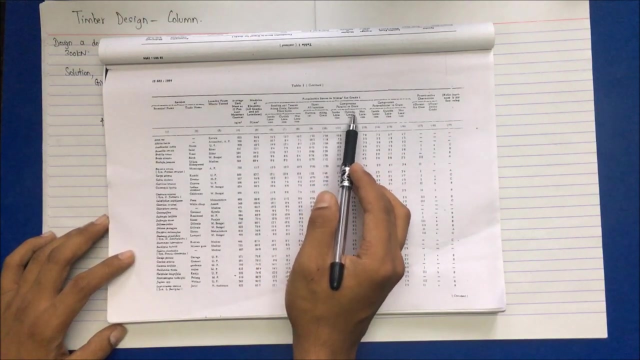 taken as 557 kg per meter cube and modulus of elasticity is taken as 94.8 into 10 to the power 2 Newton per mm square. this has to be corrected in this table. similarly, we will have to take the value for Sigma CP, which is here compression parallel to grain, and you have three condition. 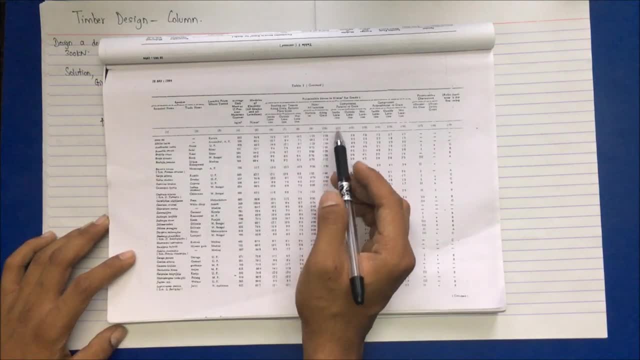 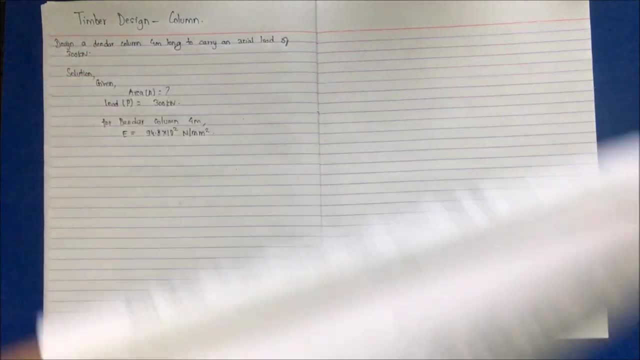 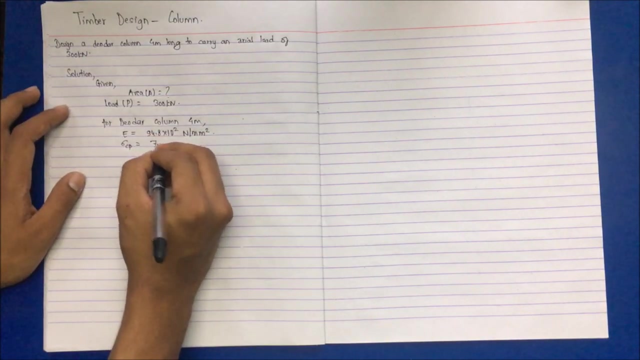 inside location, outside location and weight location. if nothing is describing question, then you will take for the inside location, and so for inside location deodorant we find 7.8 Newton per mm square, so Sigma CP is equal to 7.8 Newton per mm square. please do not get confused in code you. 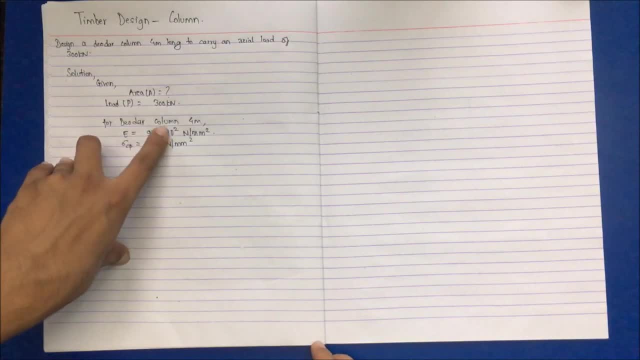 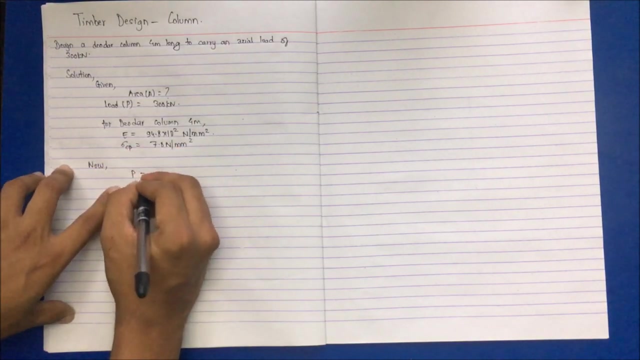 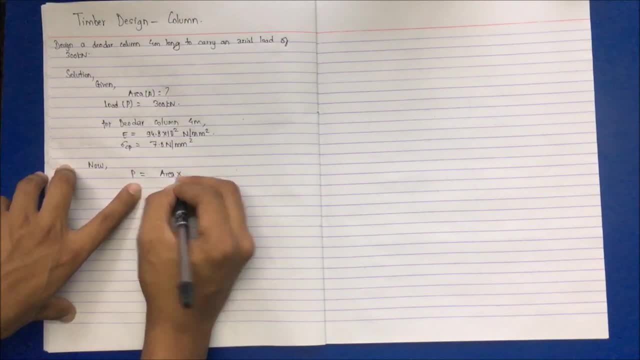 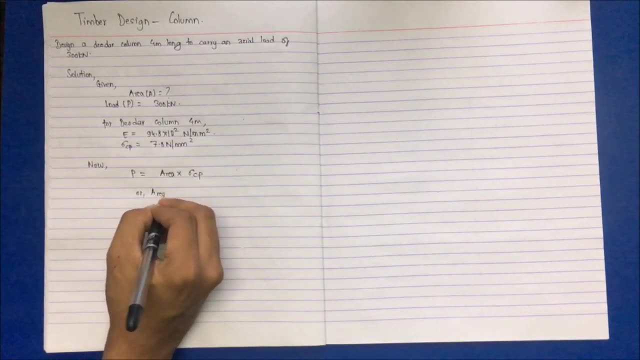 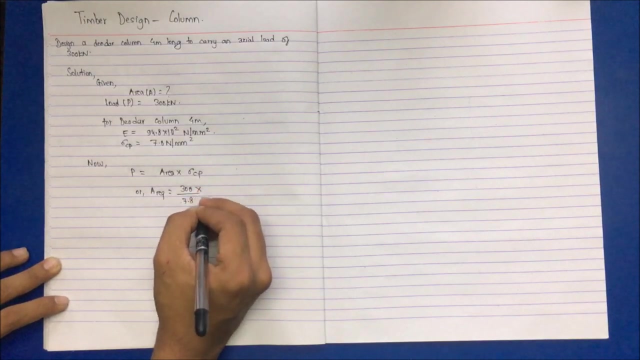 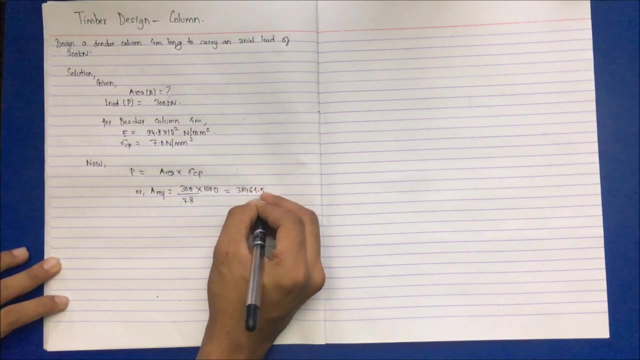 formula that load is given by area multiplied by Sigma CP. okay, then we get area required as 300 kilo Newton, by Sigma CP as 7.8. this is in kilo Newton and this is in Newton per meter. so multiplying by thousand, we get area required as three, eight, four, six, one point five mm square. 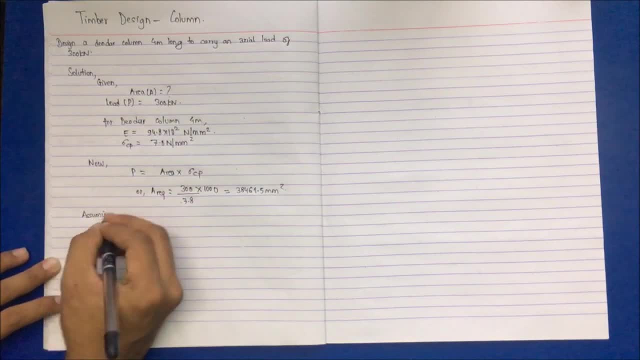 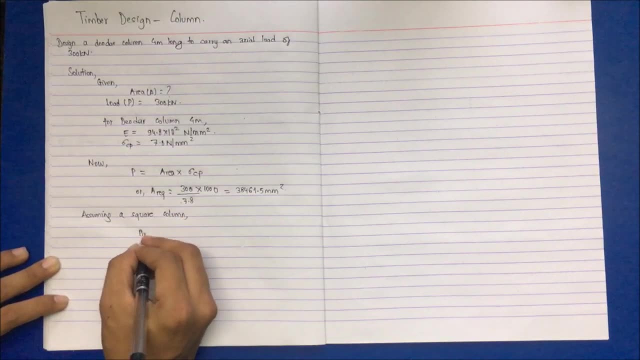 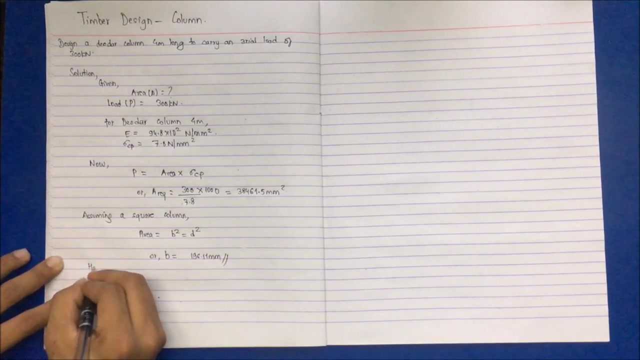 assuming this is a step you have to know, assuming I column, that means all the dimension will be same. P, sorry, area is equal to B, square is equal to D, square or B is equal to, will get, as 196 point one, one mm here provide be nearly equal to 250 mm. 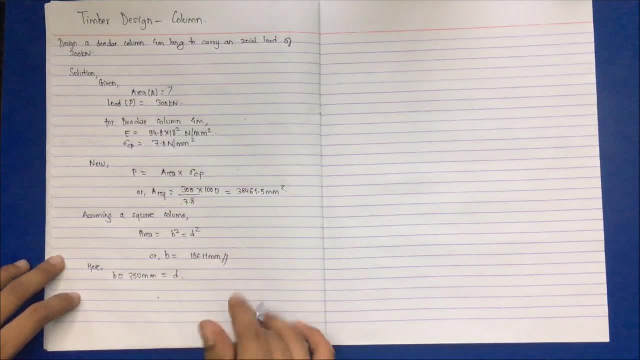 that will be equal to depth of the beam, depth of the column, so be, and we will see how we can get the height of the column also. so you have to know that. so this is the set area variable that we have of the size of the column. so you have to know that you can get the height of the column. so we will put. 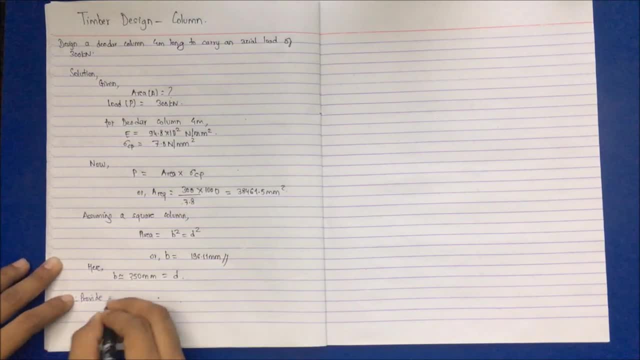 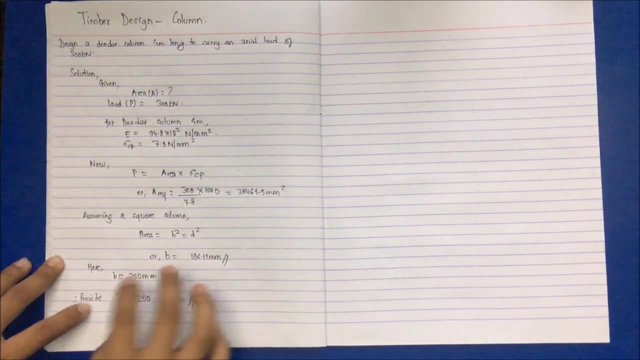 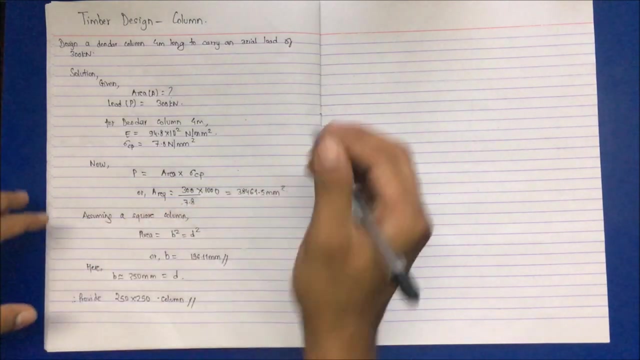 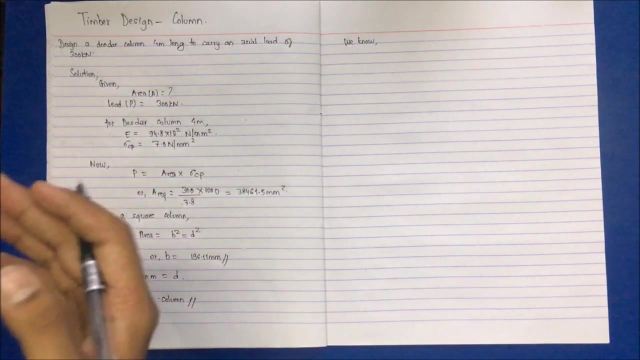 provide 250 mm by 250 mm column. this is the general procedure. now we have to check whether this is a short column, intermediate column or long column. we know. to check whether it is a short column or long column or intermediate column, we need a ratio of L by D, where L is the length, or you can find in the: 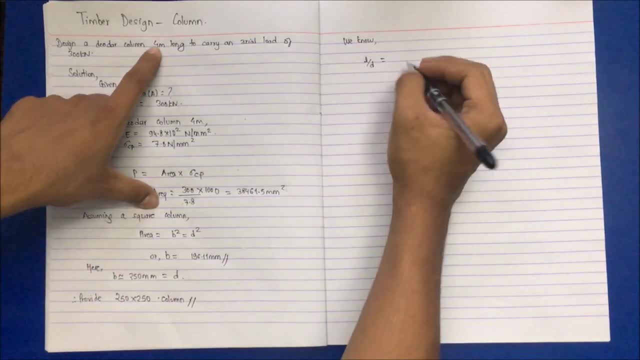 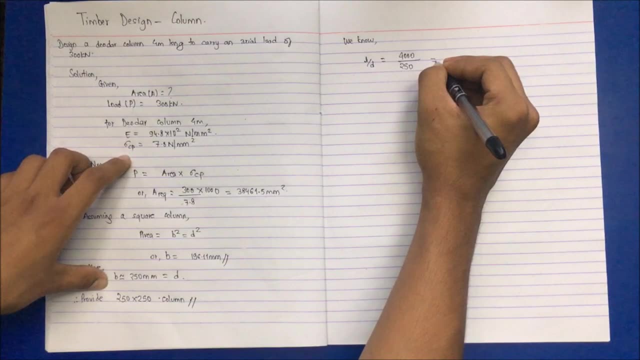 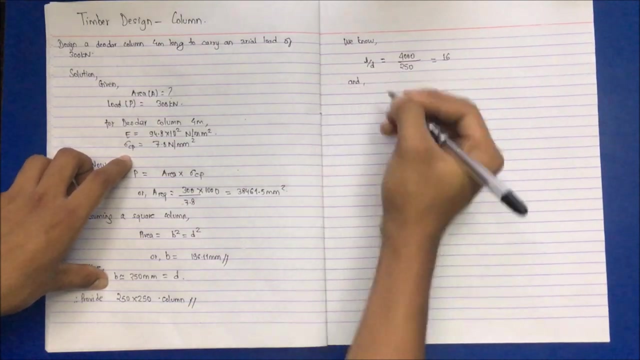 book and the code as S: okay. L by D, which is 4 meters. so keeping in mm 4000 by depth, which is 250, I get this value as 16. okay, and if you check the condition for short column it says so. this is a case of solid column. 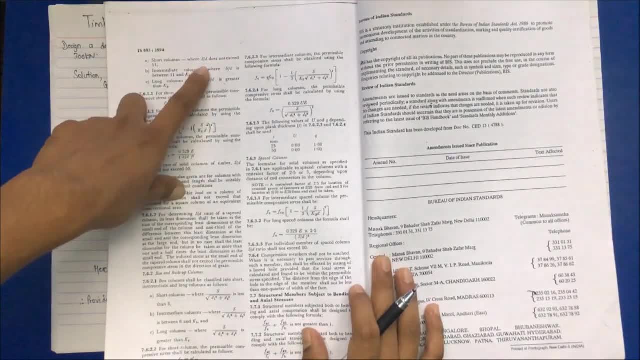 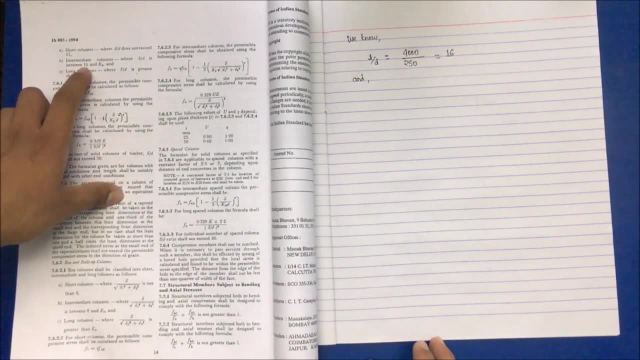 okay. if you check the condition for short column it says so. this is a case of solid column and for short column, s by S by D should not exceed 11 and our value has come 16, so it doesn't satisfy the condition of short column. and for intermediate column: 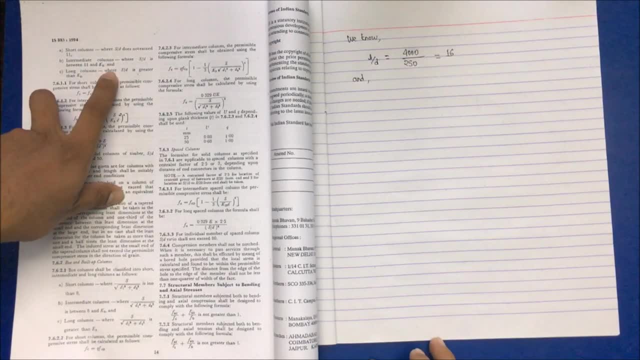 it should be between 11 and k8. k8 is a constant which we will find with the formula which is provided at the appendix. okay, and for long column, the value should be greater than 8- k8. so let us find k8, which is a constant equal to. 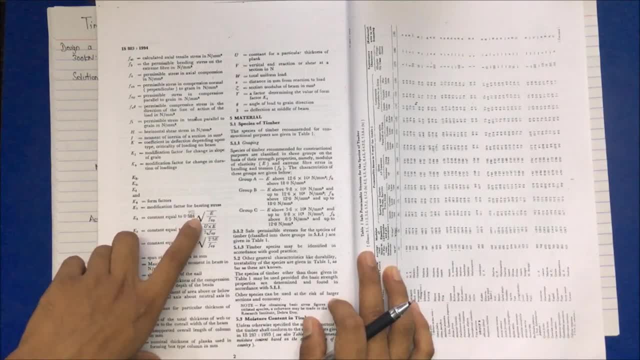 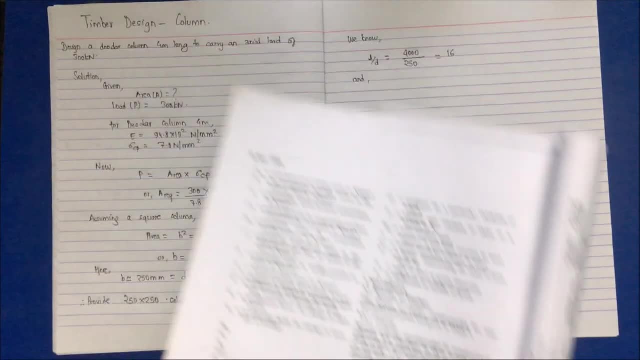 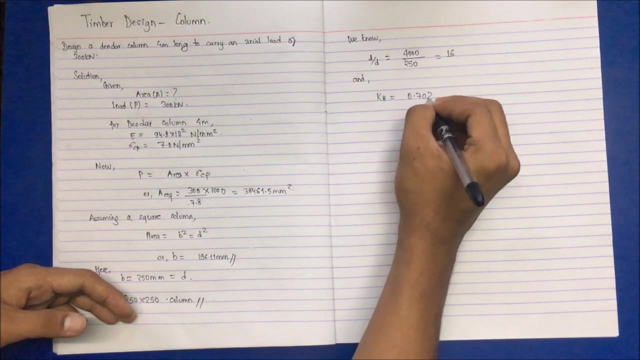 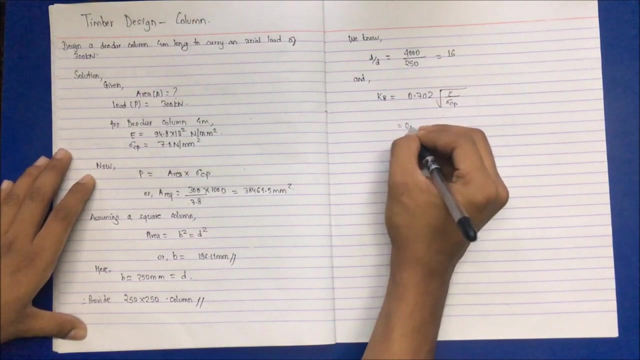 zero point seven zero two. this is a mistake in the code books. zero point seven zero two. under root e by fcp: fcp is value equal to Sigma CP. so k8 is equal to zero point seven zero two. e by the modulus of elasticity: Sigma CP. zero point seven. 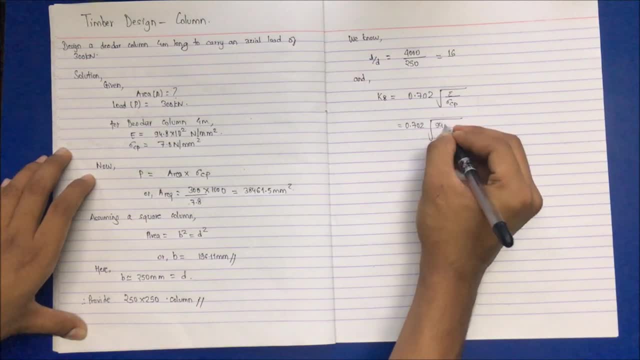 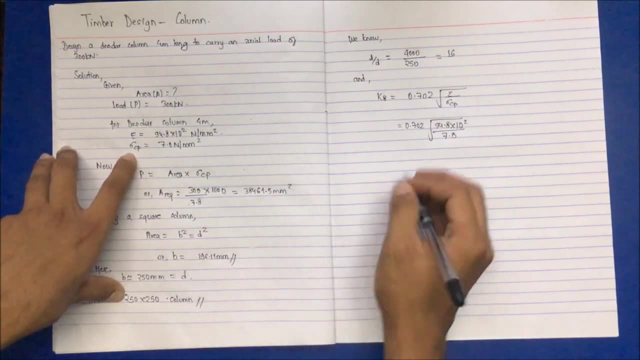 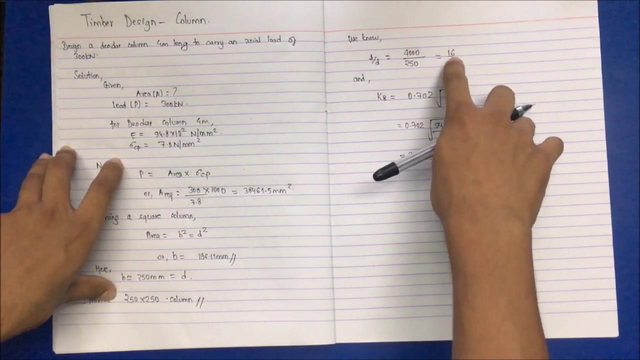 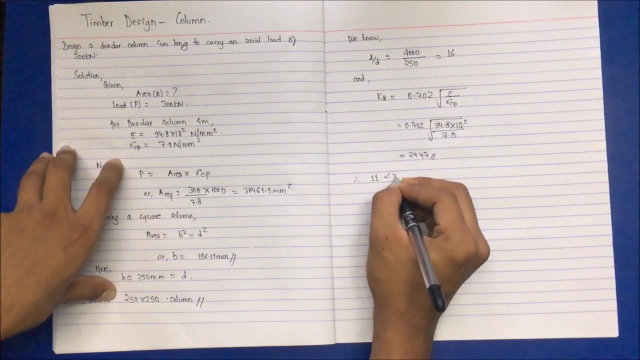 zero two e, that is ninety four point eight, into ten, to the power two by the by seven point eight. okay, we have calculated the value from the table. so this comes as twenty four point four seven, and L by D does not exceed twenty four point four, seven. that is, the value lies between eleven and twenty four. 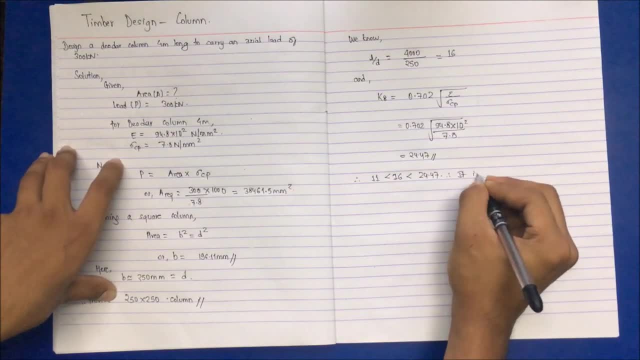 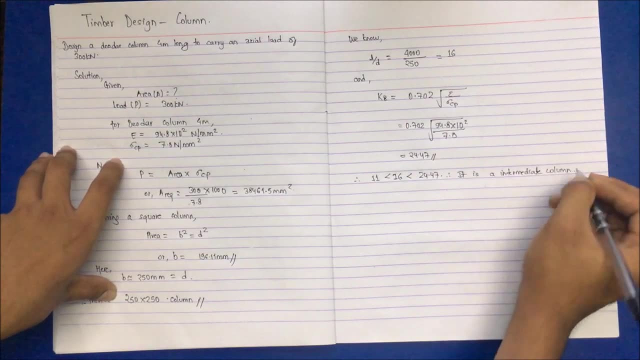 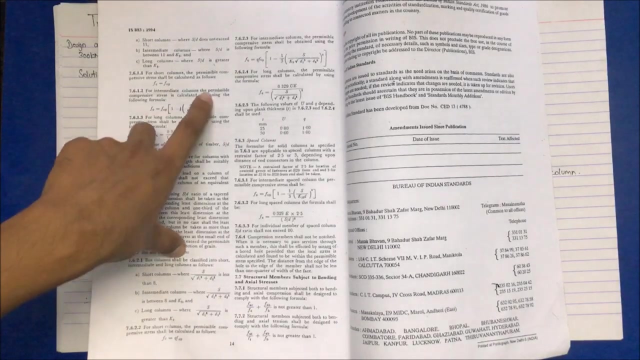 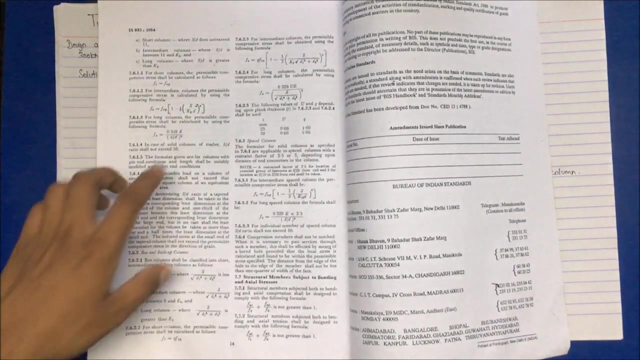 point four, seven, that is k8, hence it is a intermediate column. if it is an intermediate column, then again, looking in the code book for intermediate column, the permissible compressive stress is calculated by using following formula, that is, FC is equal to FCP, 1 minus 1 by 3 s divided by: 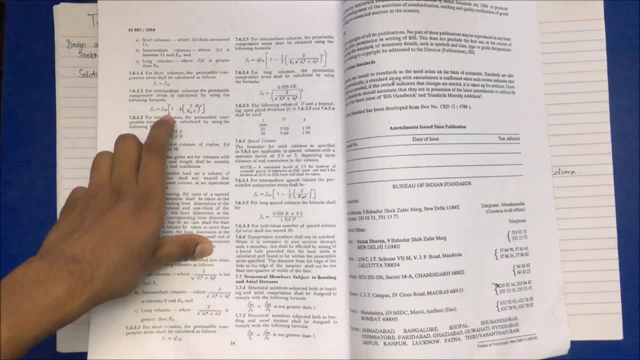 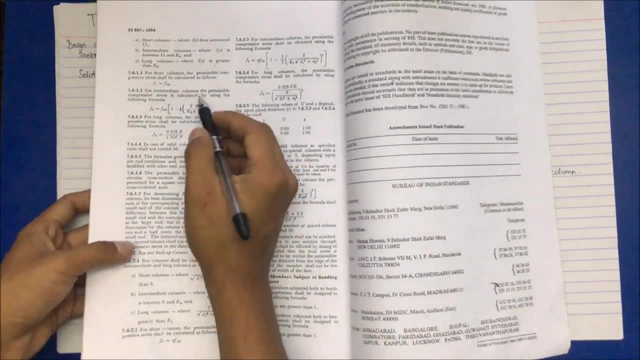 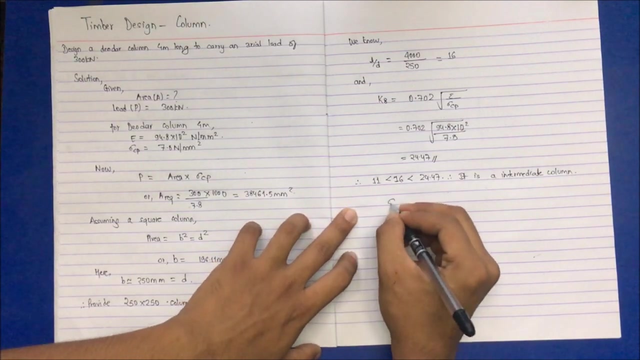 k8 into D to the power 4, so FCP, which we have taken from the table. s is the length, k8 is we have calculated and D is the depth. if we see, we have just calculated the s by d term, that is l by d here. okay, therefore, sigma, cp, dash. 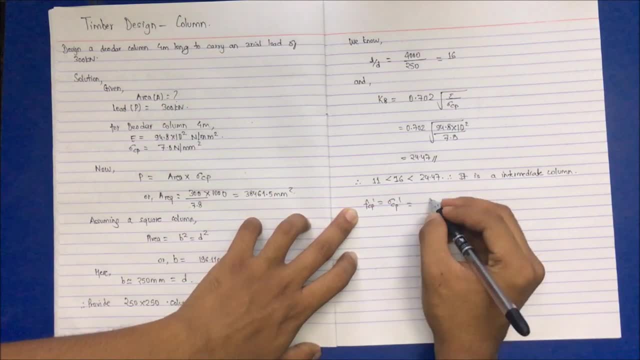 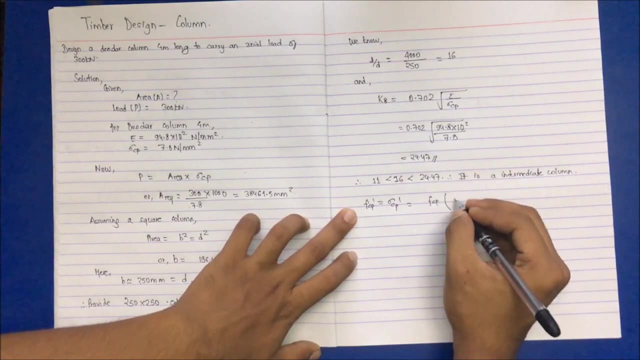 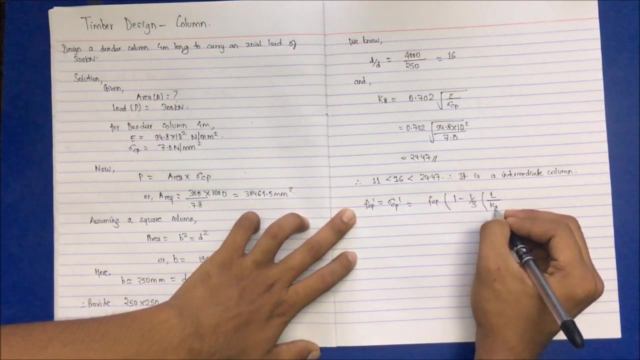 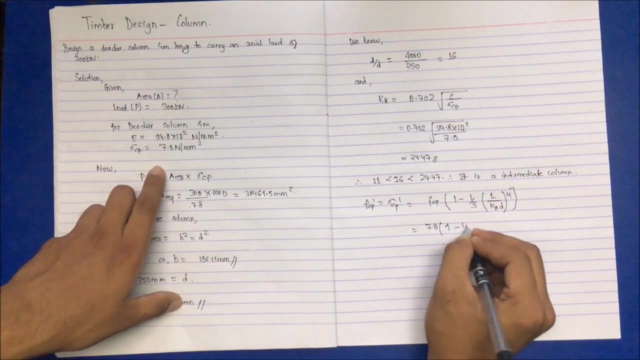 okay, in code book you find it this as sigma cp dash is equal to f cp. or you can just write a sigma cp: 1 minus 1 by 3, l by k, s, k, 8, d to the power 4.. sigma cp is 7.8, 1 minus 1 by 3.